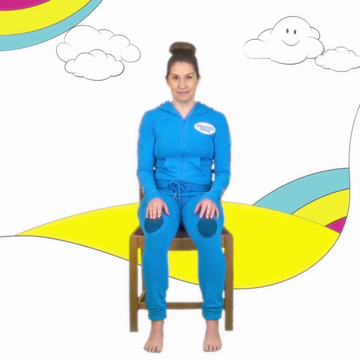 First take a seat. Now we relax. Close your eyes if you like, Breathe out and be still. Place your feet side by side on the floor. Notice them. What can you feel? Let your feet sink down into the ground. 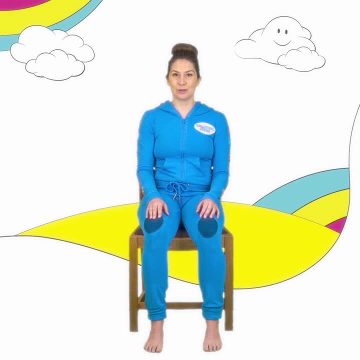 If you're wearing them. can you feel your socks, Your shoes? Are your feet hot, Cold Or tingly? Just notice your feet Here and now. Now bring your attention, like a beam of light, up to your seat, Your bum on the chair. 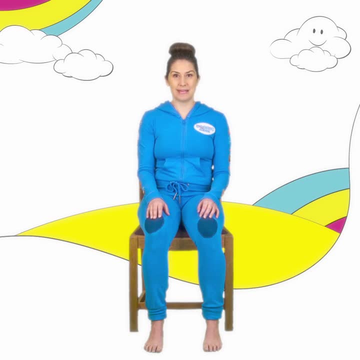 Notice the place where you and the chair meet, Feel the sensations, Just experience how your weight is held by the chair. Finally, bring your attention up to the nose, on your face, Where your breath so quietly comes in and goes out. Slightly cool on the way in. 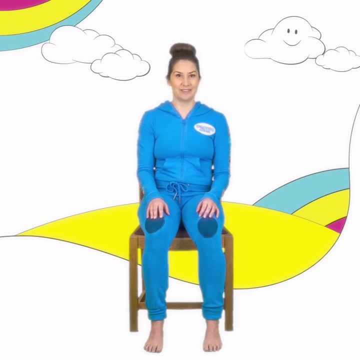 And out- Slightly cool on the way in And warmer on the way out. Just breathe. Keep your focus here for a few breaths, Noticing it moving in And out. That's all Just you, That's your breath. 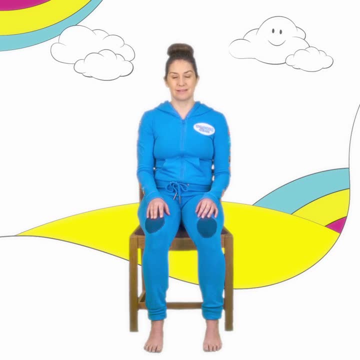 Slowly, Gently, Open your eyes. Feet on floor, Bum on chair, Nose on face. How did you get on? Don't worry if you found yourself thinking about yourself. Don't worry if you found yourself thinking about yourself.